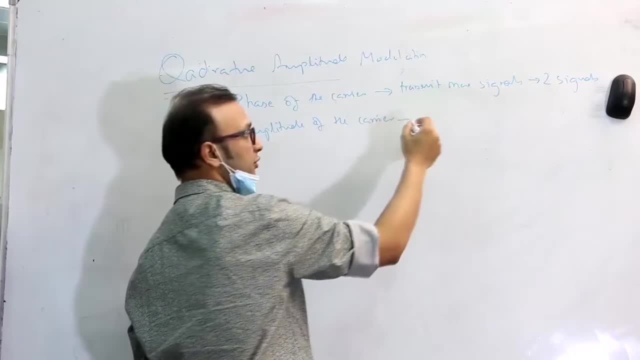 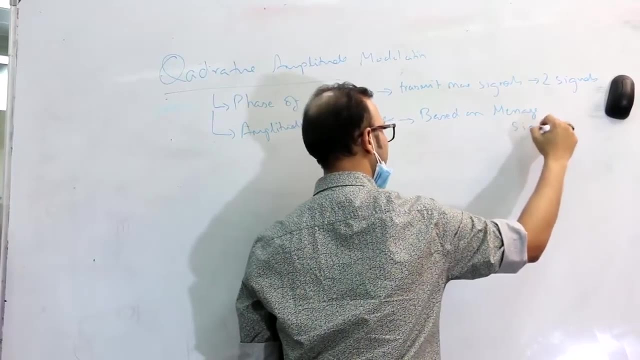 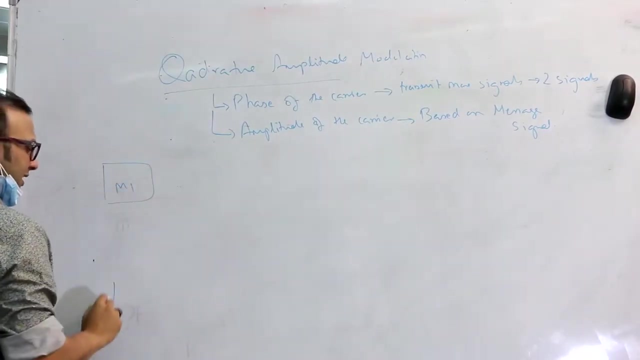 And the amplitude of the carrier will be shifted by 90 degrees. So that means you can transmit more signals And the amplitude of the carrier, of both the carriers, will change based on the message signal. Okay, Let's understand that. Let's see the block diagram. So I have message 1 and I have message 2.. Two different messages. The first message because it is amplitude modulation, so multiply with carrier. 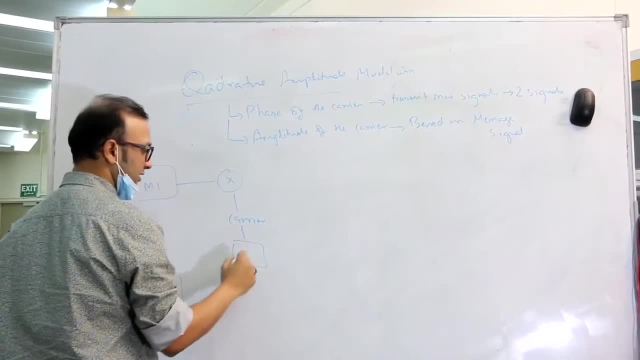 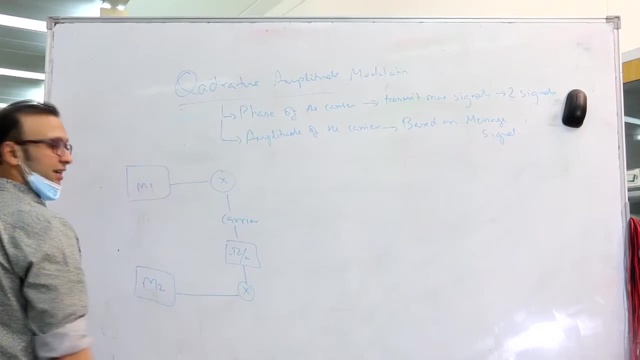 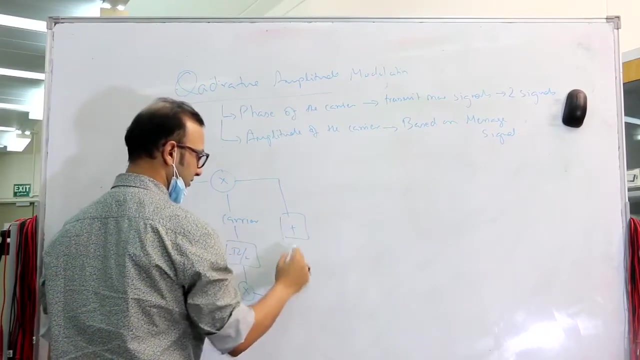 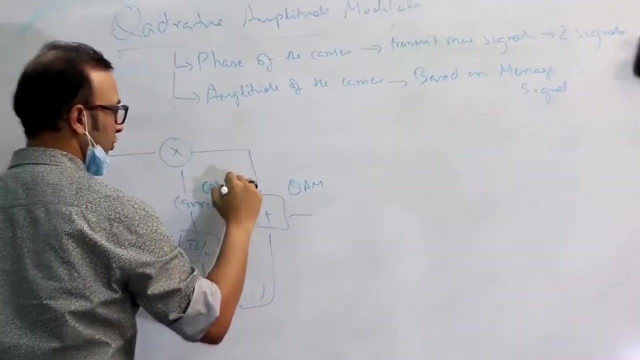 And now the same carrier is phase shifted by 90 degrees and you will again multiply the second carrier And both of them are then added And this is your quantum signal. This is cosine omega ct, And you need to do cosine omega ct minus pi by 2. You will get sine omega ct minus pi by 2.. 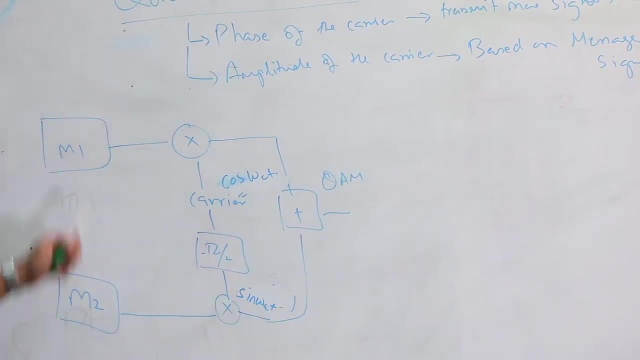 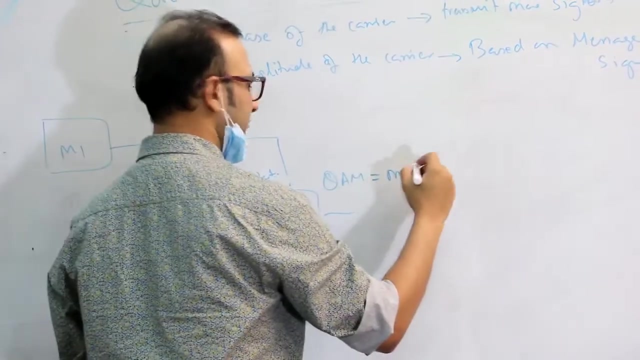 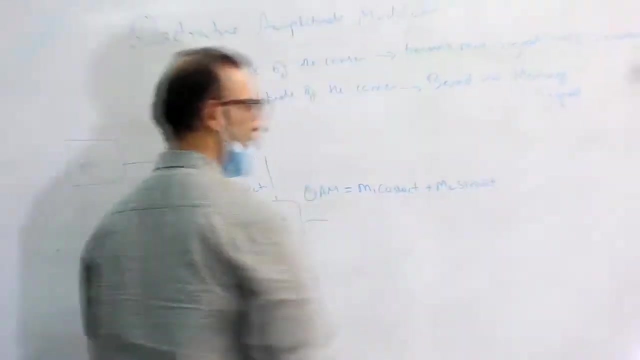 Omega CT. okay, so message 1 multiplied with cosine, message 2 multiplied with sine, so QAM signal: if you look at mathematically, it's m1 cosine Omega CT plus m2 sine Omega CT. right now I will, you will have to find the Fourier of. 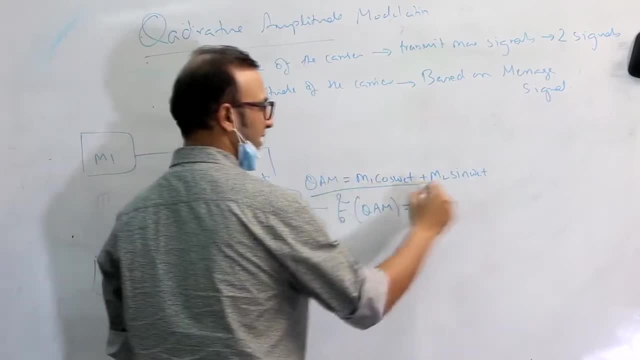 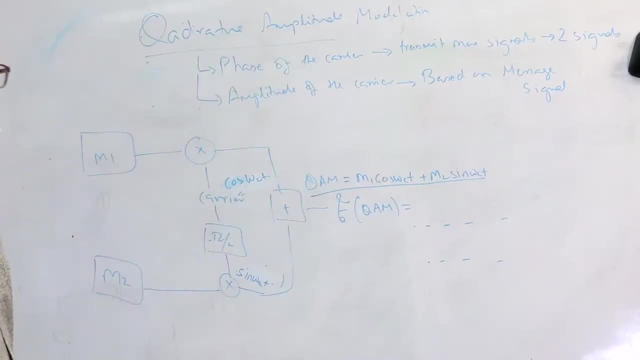 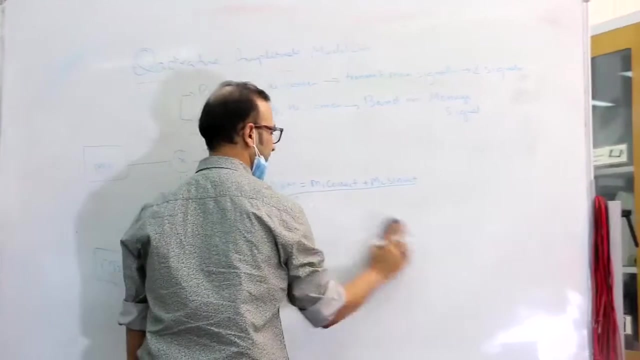 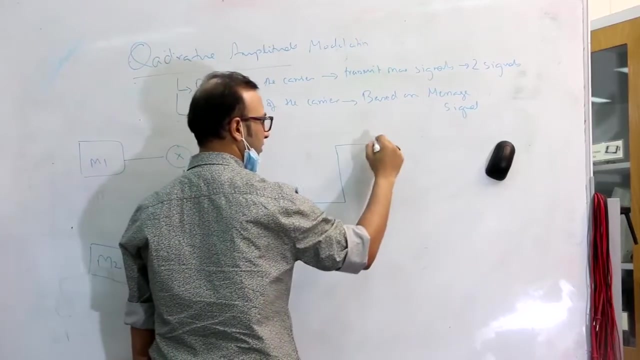 that Fourier transform of that, and so this is how it looks like in time domain. please see how it's going to look like in frequency domain. okay, so that should be in your report, all right. okay, let's go to the demodulator now. in the demodulator side, the whole QAM signal will be again multiplied with the same. 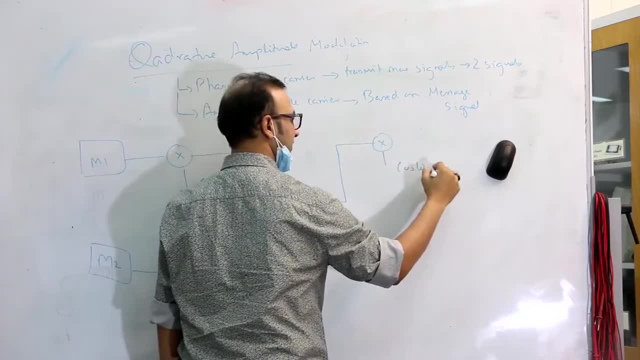 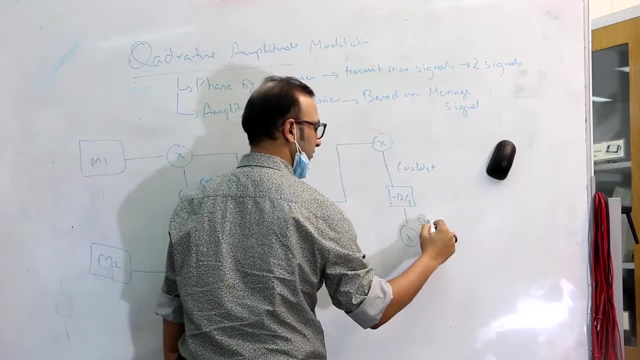 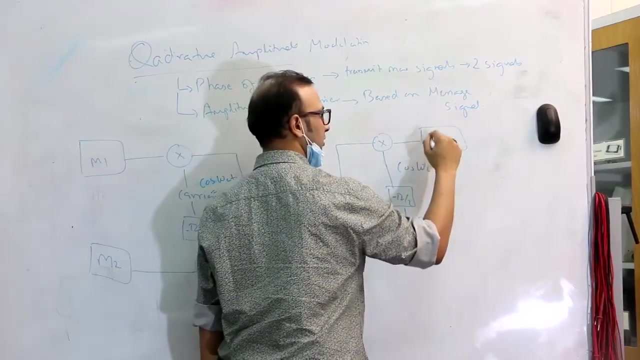 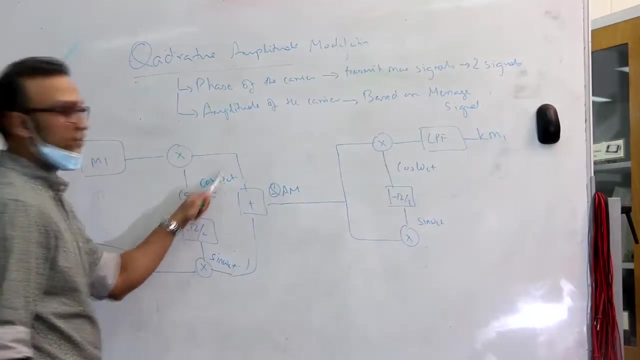 carrier cosine, Omega CT, which is again phase shift it to give it the second carrier right, and then this pass through a low pass filter to give you a scaled m1, because m1 must multiply by cosine. so in the demodulator side the same Omega CT is multiplied with the QAM signal and then 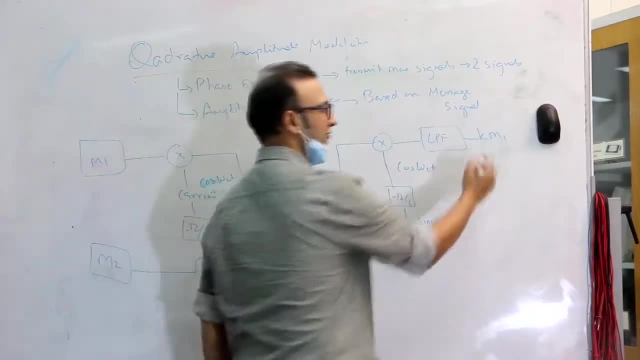 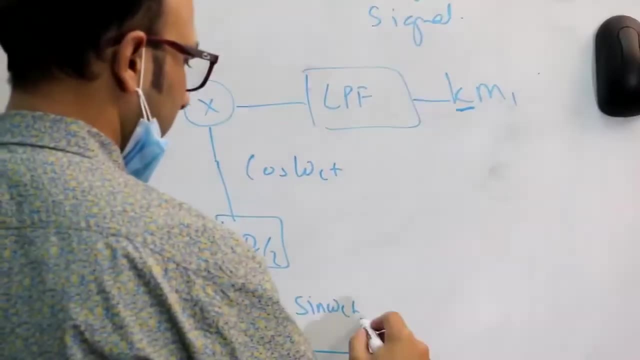 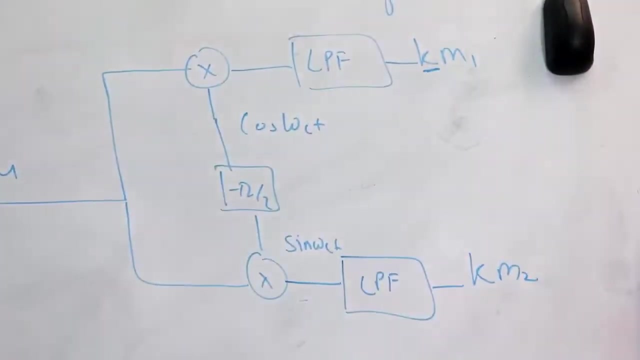 pass through a low pass filter, you get scaled version of m1. scaled means it can be half over kanjik. we can see that right mathematically. similarly, when this group of the power filter, you get scale and two. okay, now, at any point of time, for 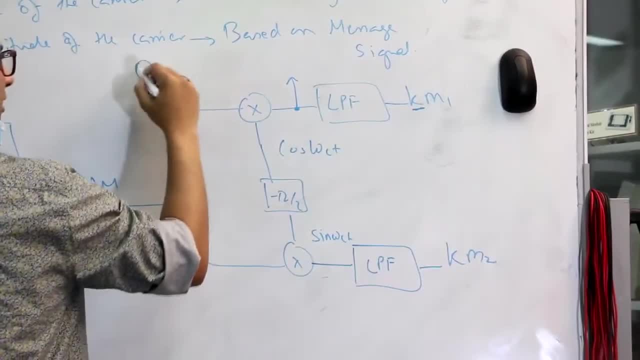 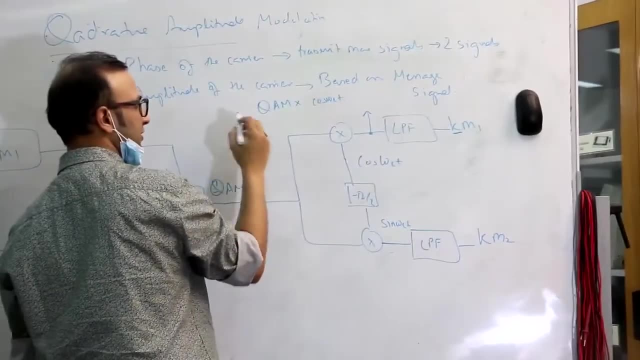 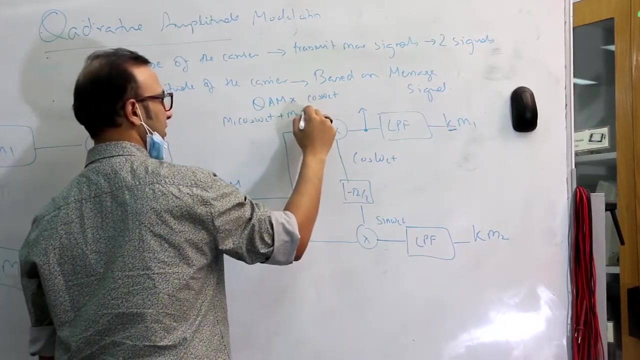 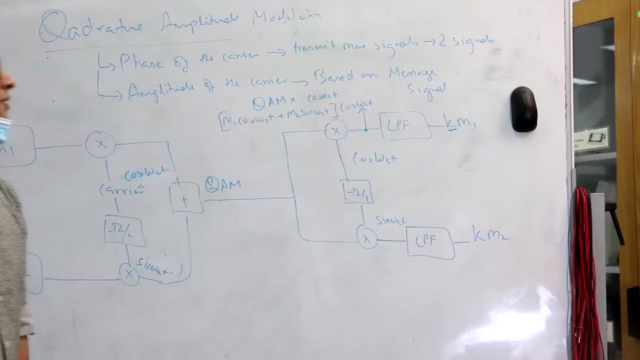 example here. if I need to know what is my signal, it's QAM signal multiplied by cosine Omega CT. so that's again we know what the problem is. so QAM is m1 cosine omega CT plus m2 sine omega CT, the whole multiplied with cosine omega CT all. 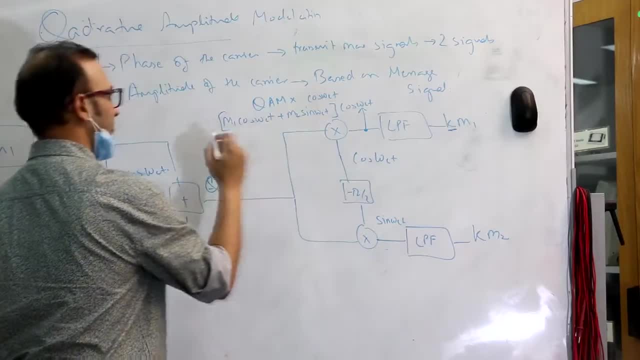 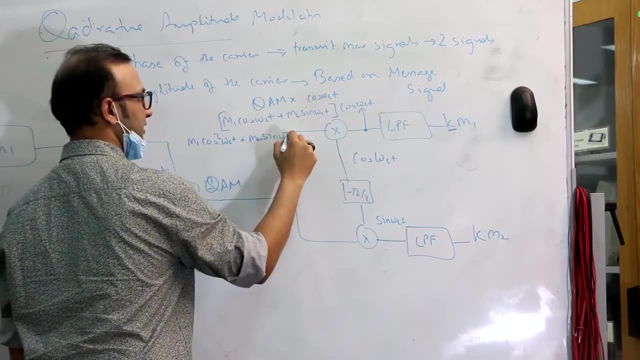 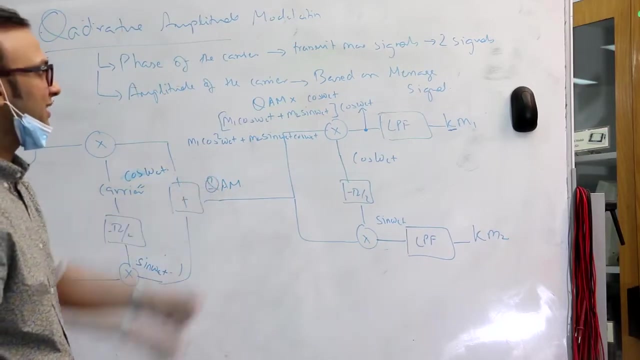 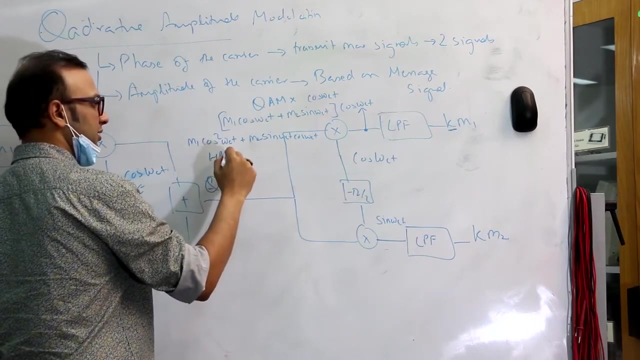 right. obviously you will have something like this: m1 cosine square omega CT plus m2 sine omega CT- cosine omega CT. right using the trigonometry functions, you will see that at the end we will have some high frequency components and then low frequency components which, when passed through a low pass filter, will. 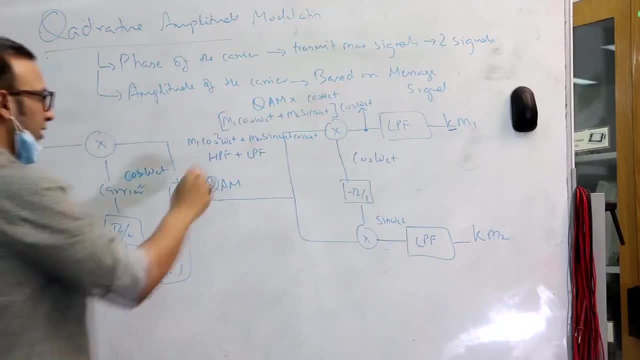 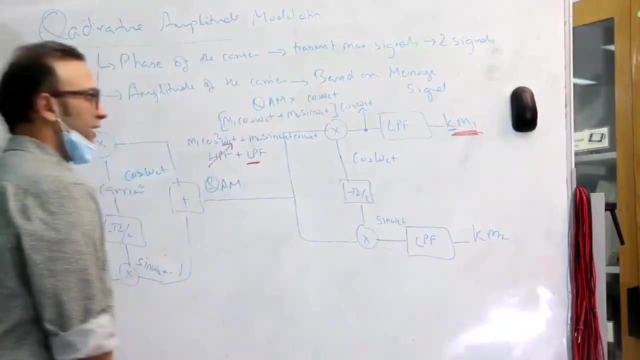 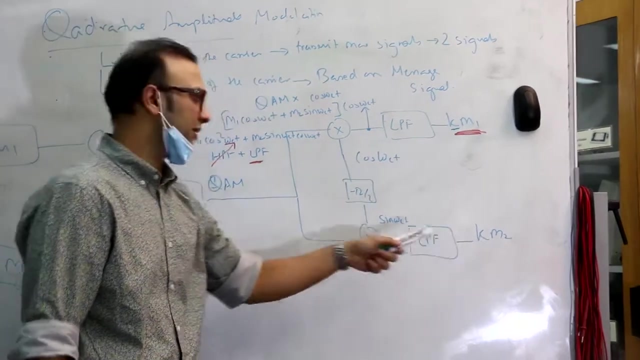 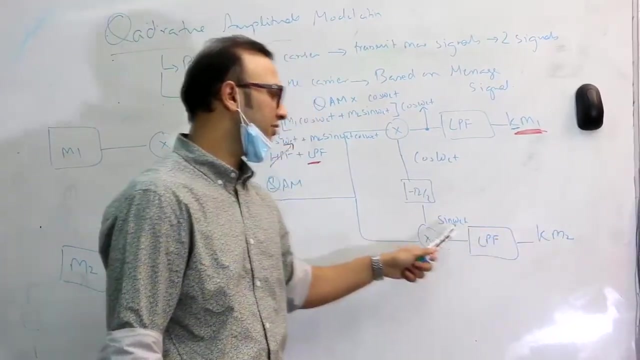 get rid of these high frequency components and you're left. you will be left with the low frequency signal, which is m1. okay, all right. same thing happens over here with sine omega CT. if you do the math again and then pass it to a low pass filter again, the high frequency component goes away and you're left with 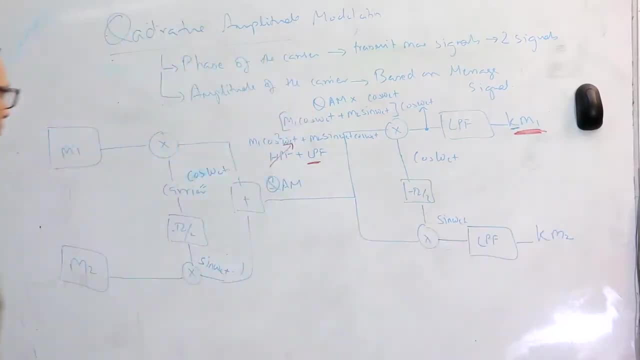 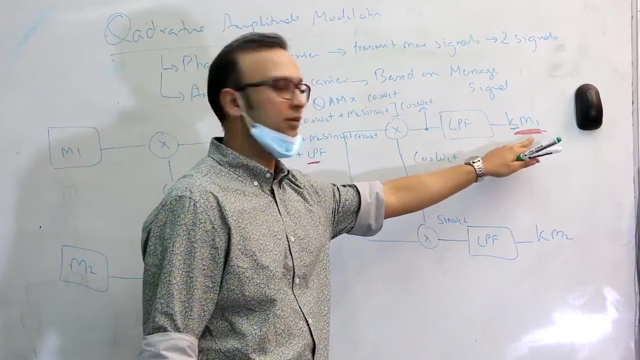 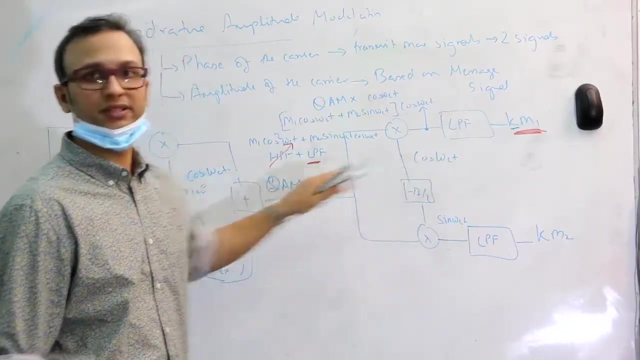 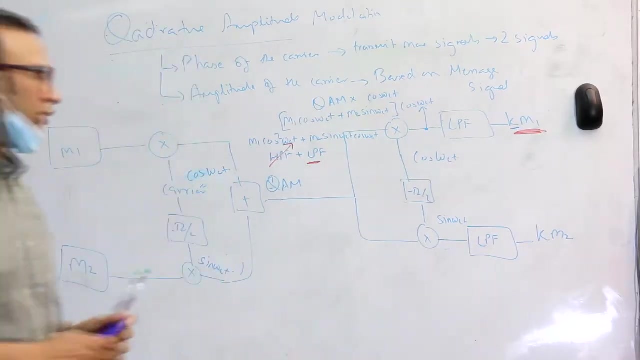 only m2. so, as you can see over here, we are transmitting two signals and at the end we are getting back the same signal back. we are getting the signal, the desired signal, by just multiplying with the respective carrier frequency. one thing you have to be, you have to take care, is we should always avoid, suppose, if there is any sort 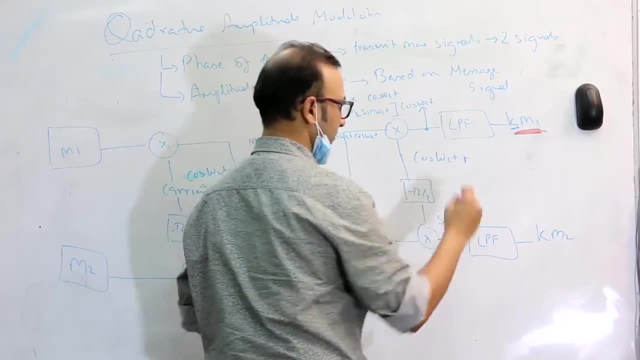 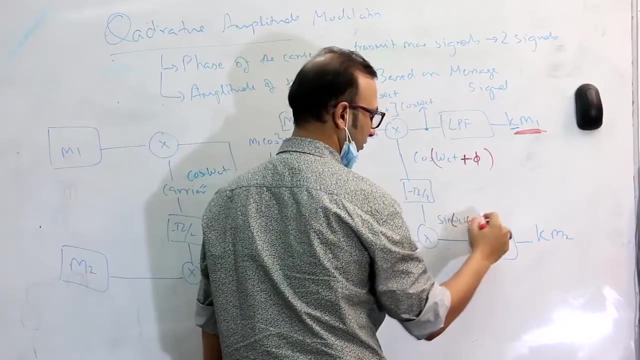 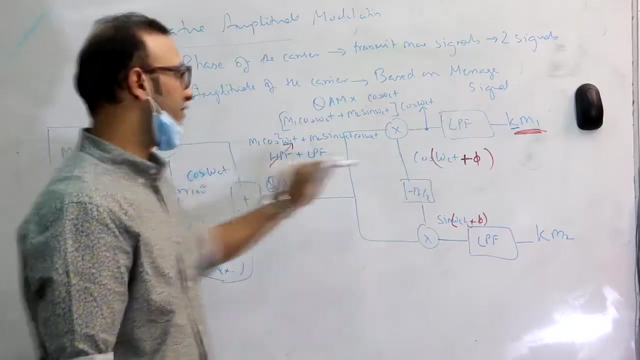 of phase shift. if there is any sort of phase shift here or here, okay, over here there's a phase shift. that means it's not the same carrier that is multiplied, it's a carrier with a phase shift. then you will not. you will not have KM1 alone. 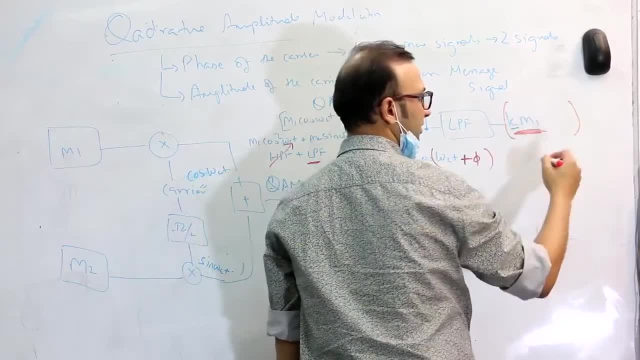 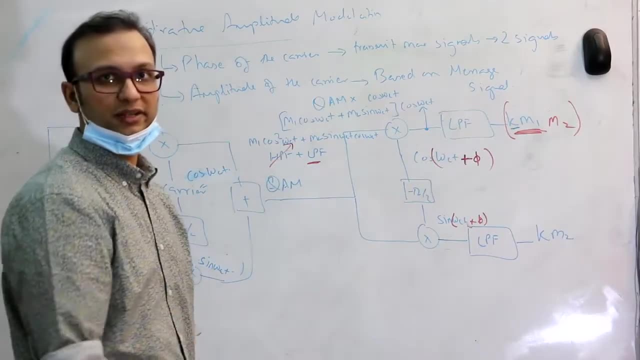 you will have a M1 and a KM2, one a distorted signal, so you will have also m2 here. okay, obviously you have to do the math all right, or do the whole formulation thing. this should be there in the report. same thing: if there's a phase shift over here, then you will have. 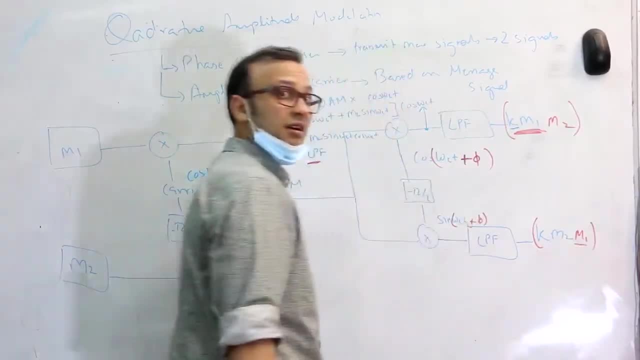 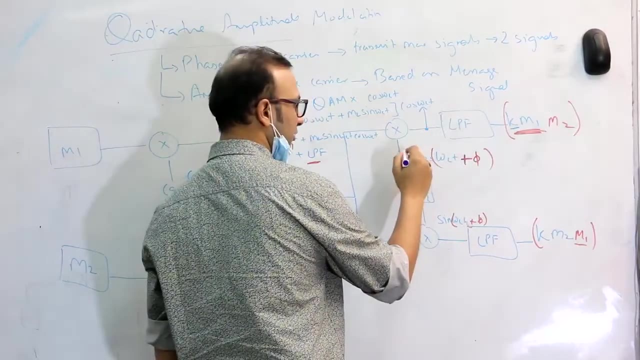 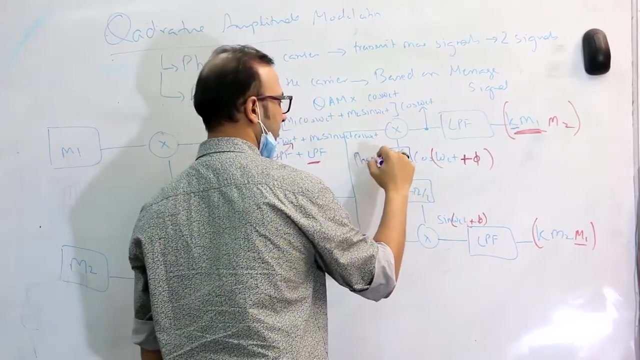 K and 1 into. as you can see, there's interference now, so that the best way to fix that is when it, when you are multiplying it, have a phase shifter. this is called as a phase shifter, and this phase shifter will get rid of the extra. 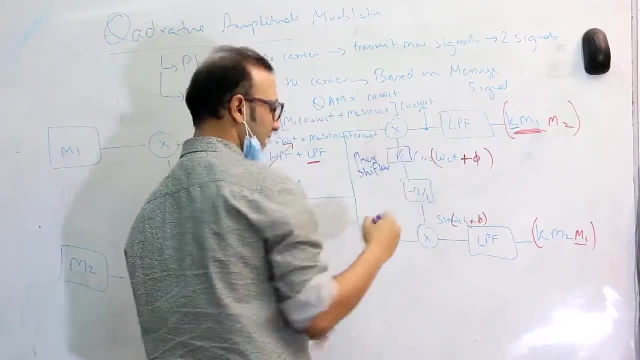 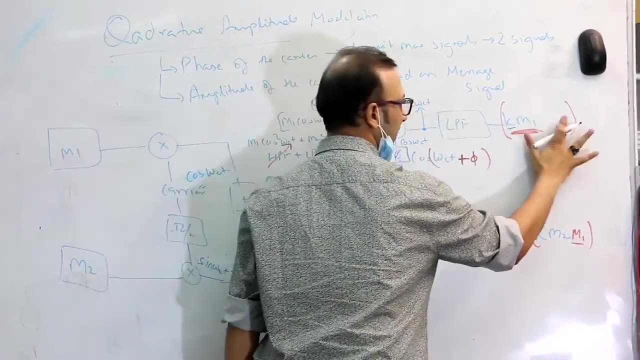 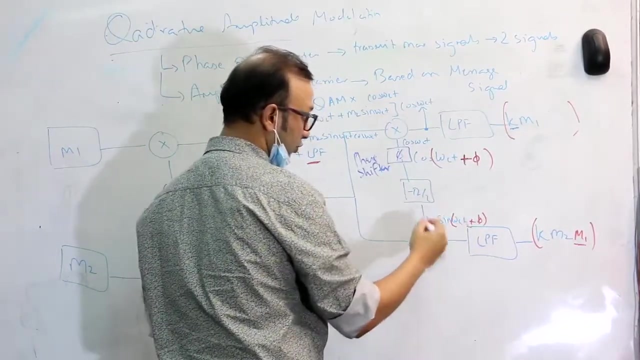 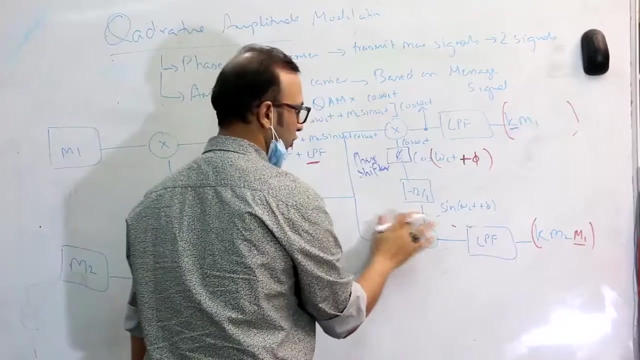 phase that is there. so if you remove that phase and at the end you will be left with cosine Omega CT and then you will not have this extra interference. similarly over here again before it goes, so let me write it over here: it's plus five, so you: 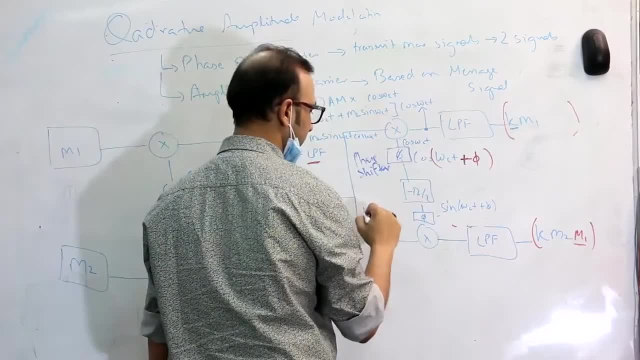 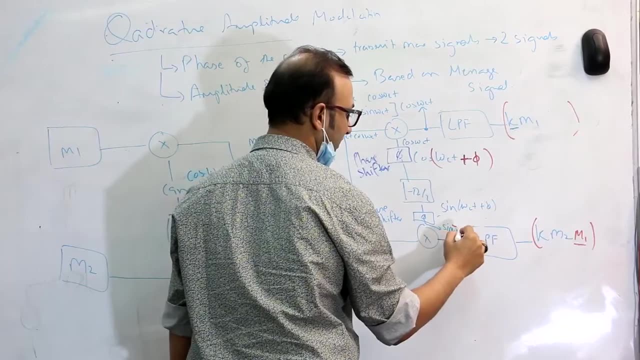 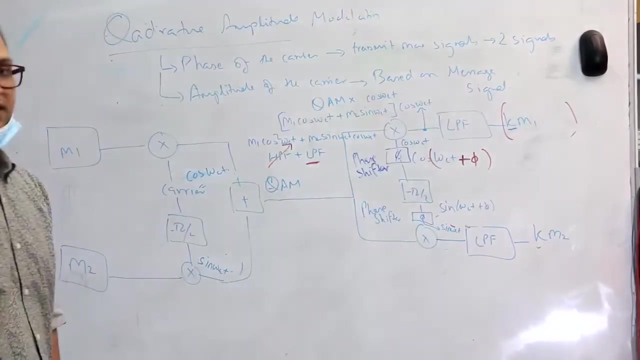 will have again a phase shifter here which will make sure that what you're multiplying is sine Omega CT and at the end there will be no interference right. so that can be easily seen when you do it in the same way. okay, we have seen how to do that in. 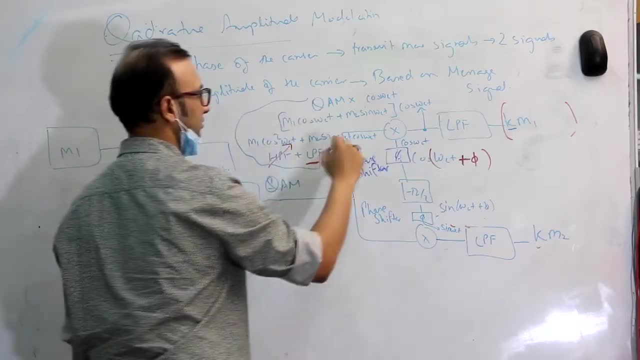 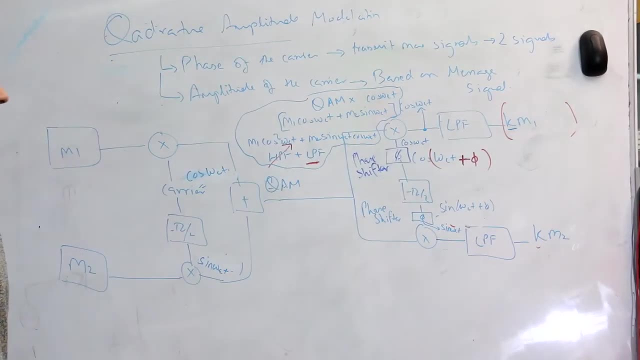 in our previous labs, right, so that would be something that should be there in the report. okay, it's also there in the videos. you can refer to them. all right, so this is what our cam modulation and demodulation looks like. now we'll go and look at it physically. okay, guys, so now we have the whole module set, I'll go. 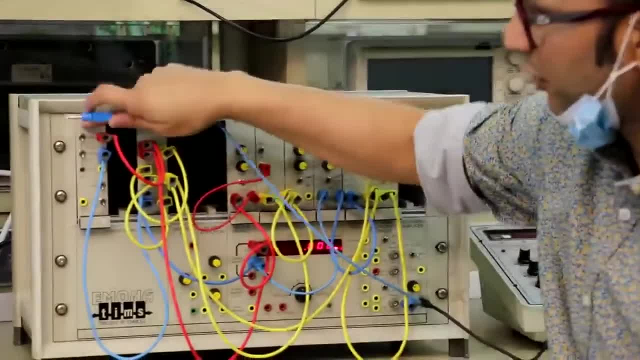 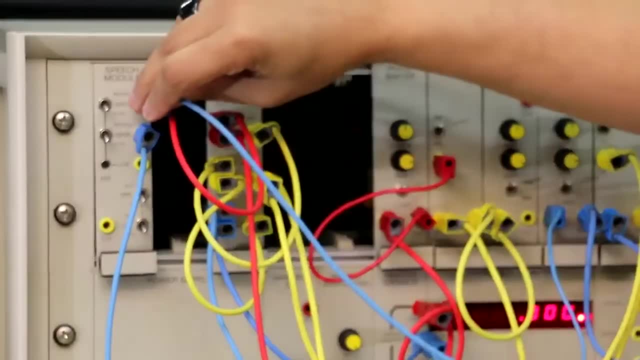 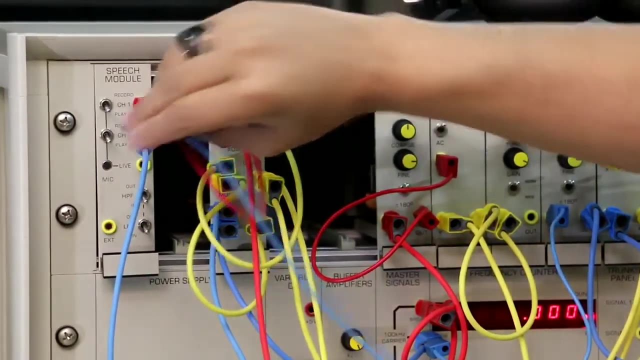 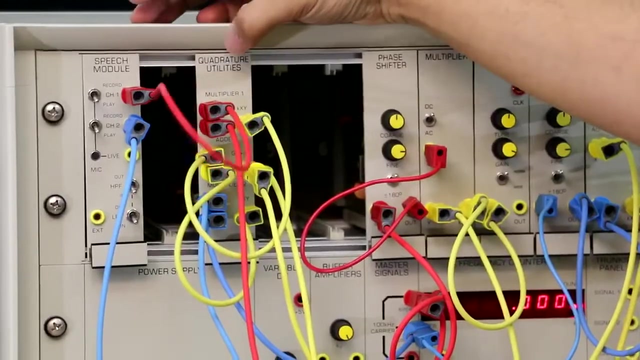 let's go through them step-by-step. my speech model and I have two signals. let's here to them my first message and the blue is mine. honest, alright, so now what I'm going to do is the first message is multiplied. this is a quadrature utility, so it has two multiplier. two multiplier multiplier one. 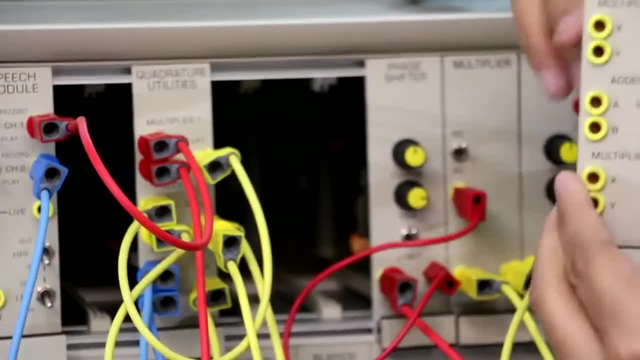 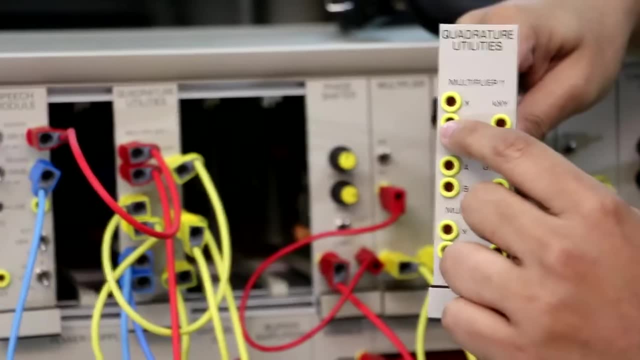 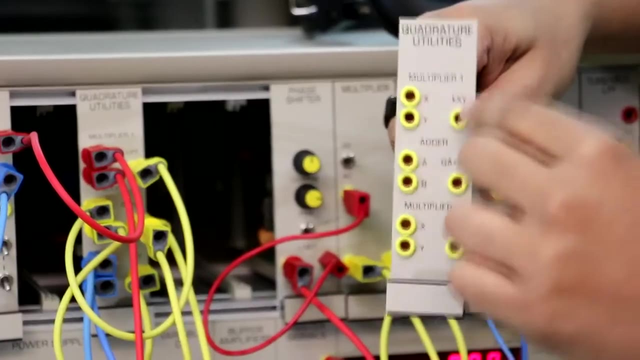 and this multiplier, two at the bottom. this is the quadrature utility. as you can see, it has two multipliers right. so this will be the signal and the carrier. this will be the second signal and the phase, like 90 degree phase shifted carrier and the output of the multiplier goes into the adder. output of this goes to the adder. 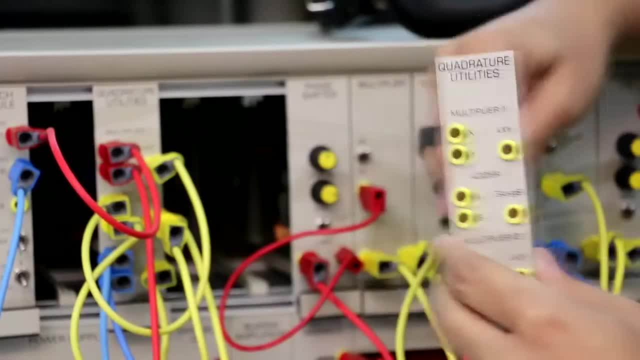 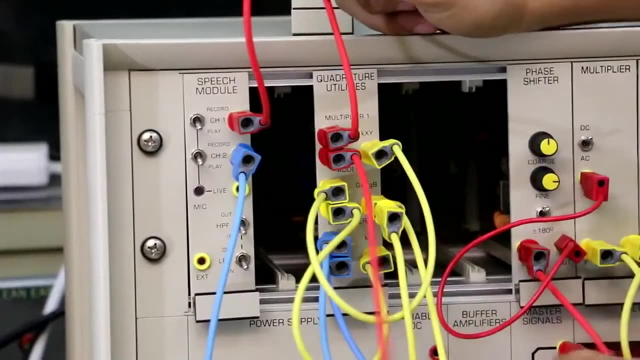 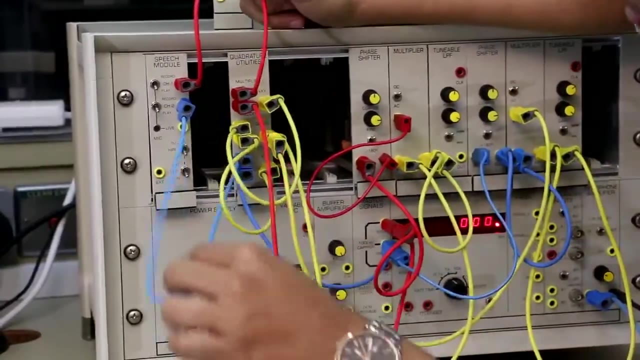 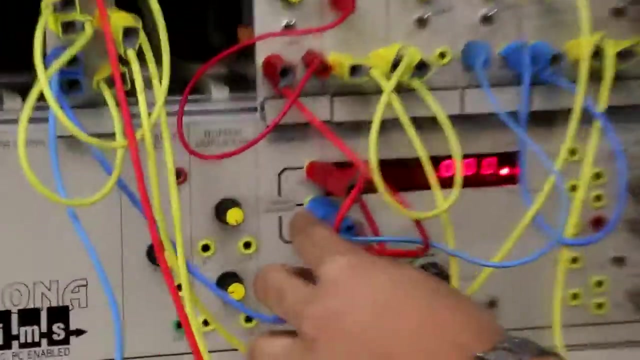 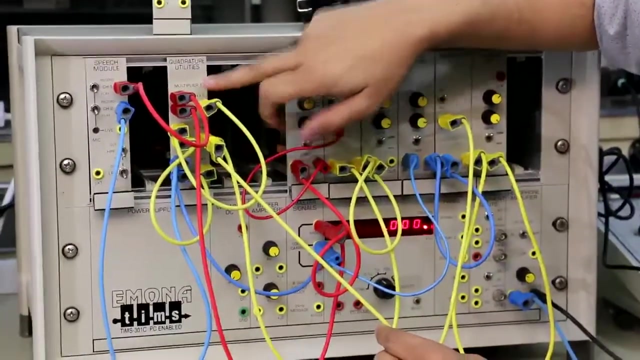 and the final output is my QAM signal. so that's what I did over here, so that's my message. one multiplied with sine, okay, high frequency sine signal. and then message second: signals multiplied with 90 degree phase shifted cosine, and then this is the multiplier output: one and 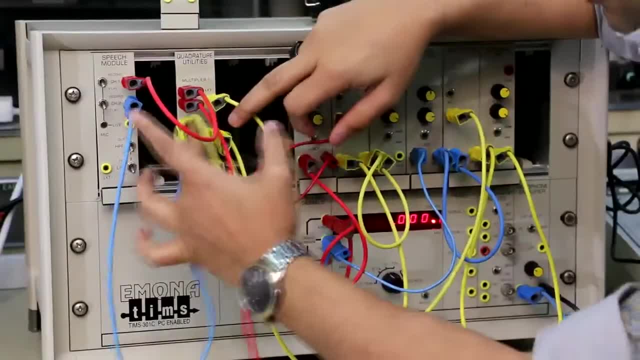 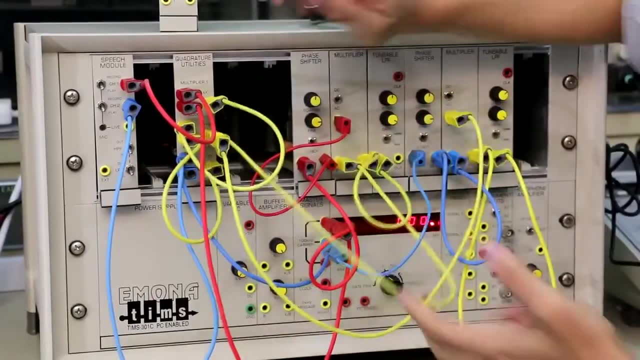 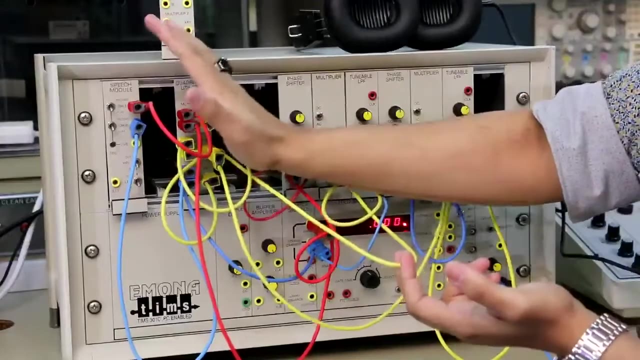 this is multiplied by output two. that goes to the adder and this is my ğı adder output, which is my QAM signal. all right, now I'm taking the first, I'm taking the QAM signal as an input to now. this is my modulated signal. now I'm this is my demodulator. so in 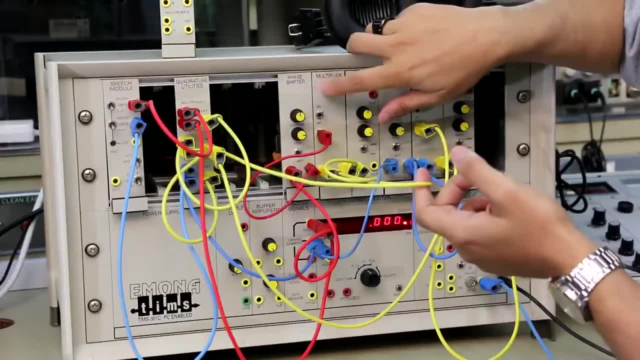 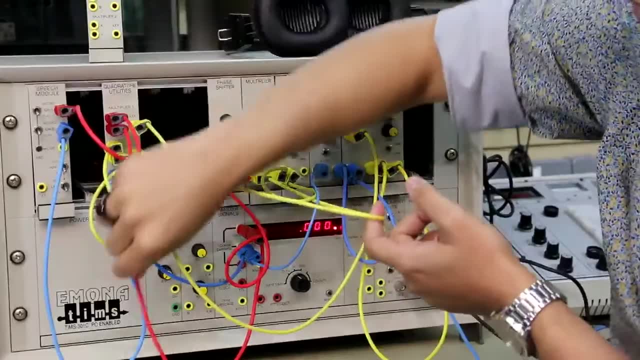 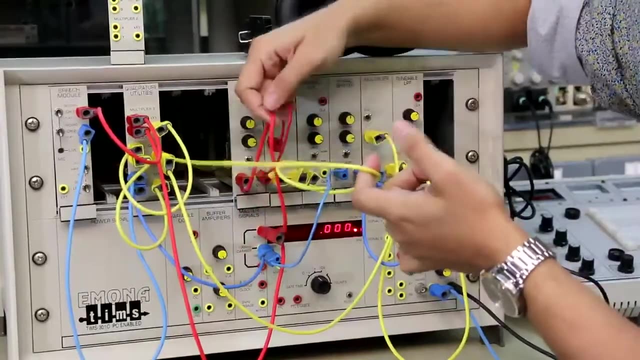 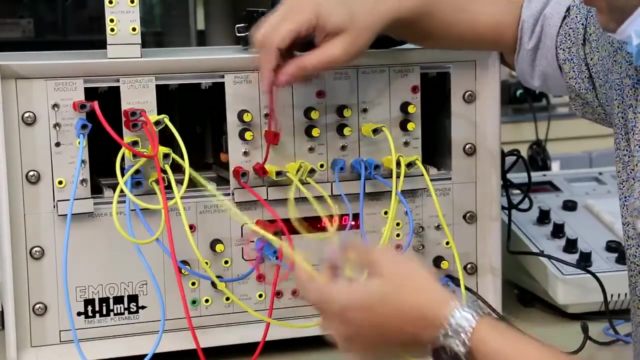 the demodulator side, the QAM signal is going to a multiplier and it is multiplied with, because I want to get message 1 which is multiplied with sign. so my QAM signal is multiplied with a phase shifted sign signal and we'll see the effect of the phase and then that signal. 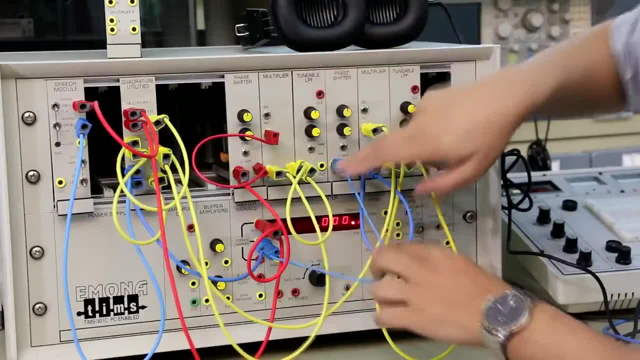 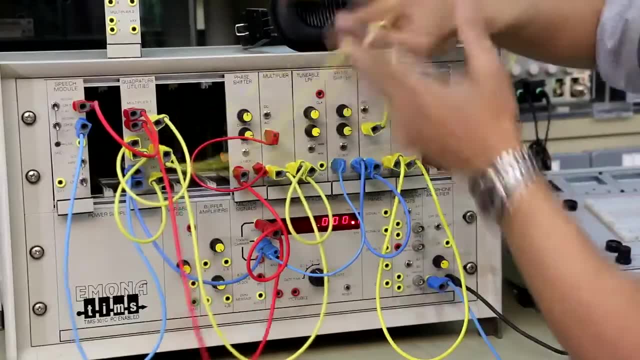 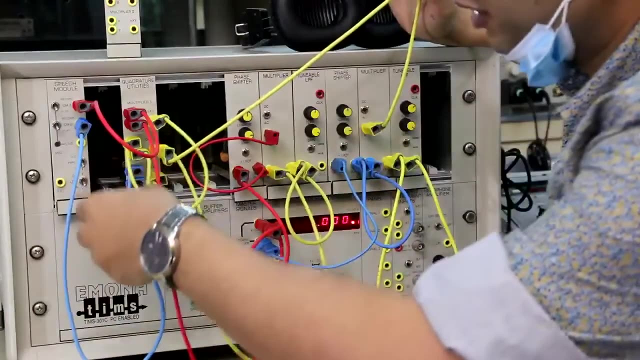 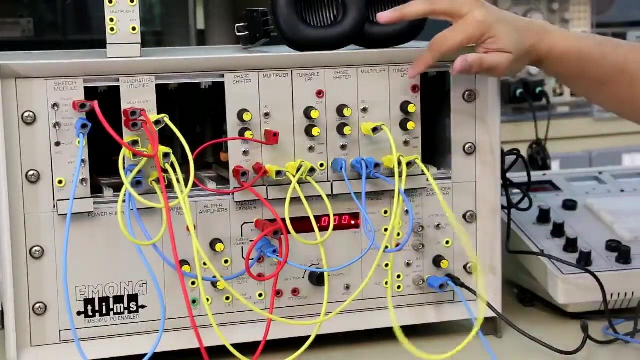 goes through a low pass filter and then- so this is my message 1. same thing happens for message 2. the QAM signal is multiplied with phase shifted cosine signal, because in the modulator side I'm multiplying with cosine, and then that is passed through a low pass filter. so let's listen to it now. 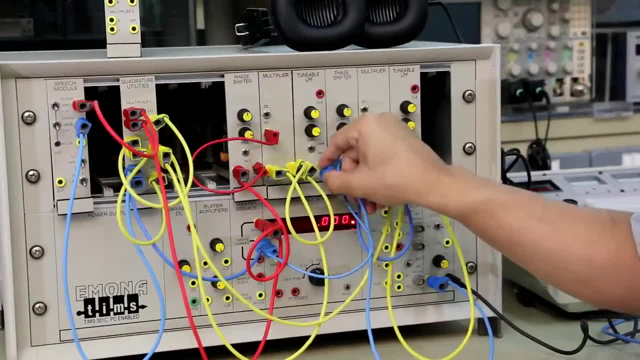 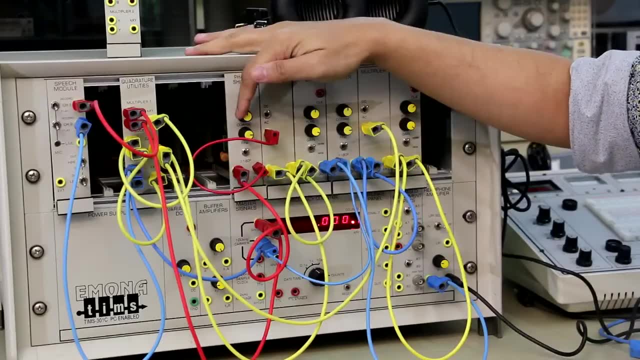 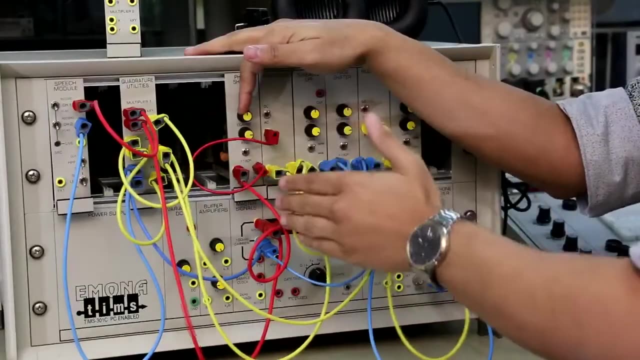 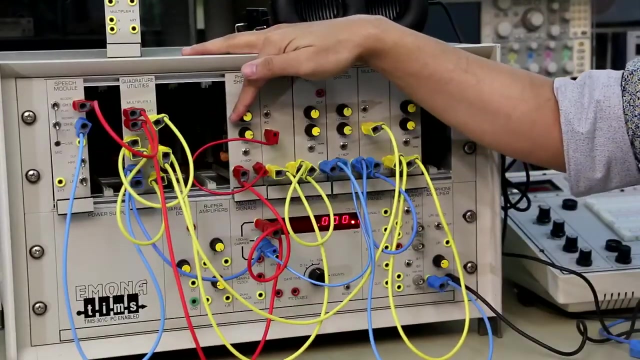 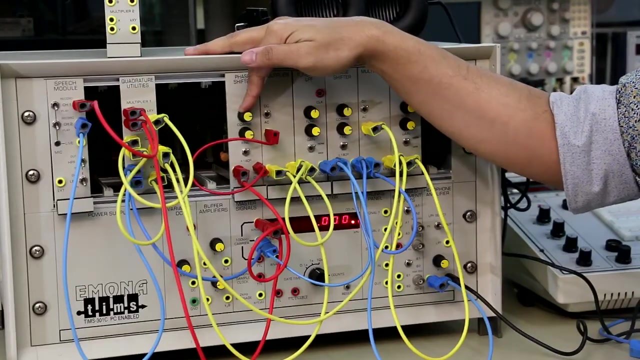 so that's my first message. right, no interference, right. but what if there was some phase difference between the carrier that was using the used here? What if there was a phase difference between the carrier that was used here and the carrier that is used here? Let's see the effect of it. You see, there is an interference. 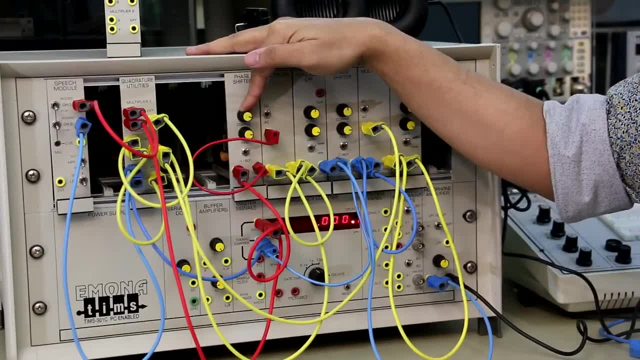 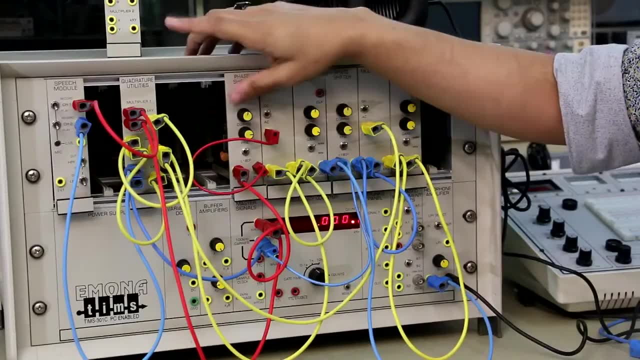 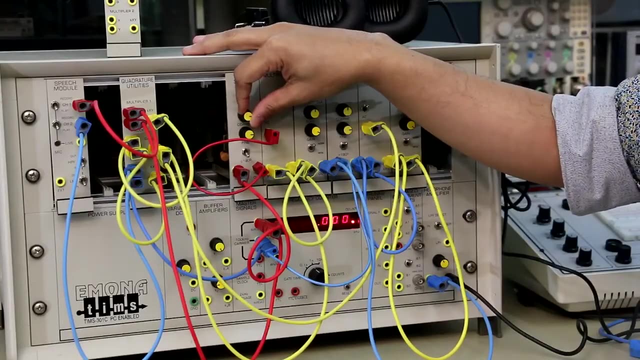 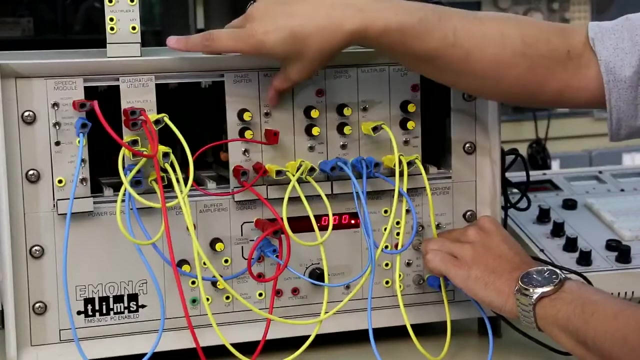 So if you want to fix it, I have to do a phase shifting. So you see there is an interference. So if the phase, if the carrier that is used here and the carrier that is used here have some phase difference, it's going to cause interference. 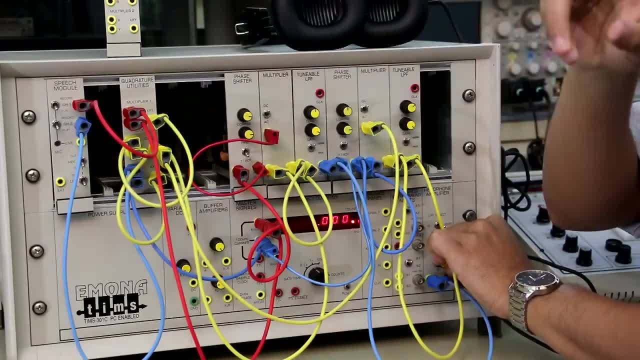 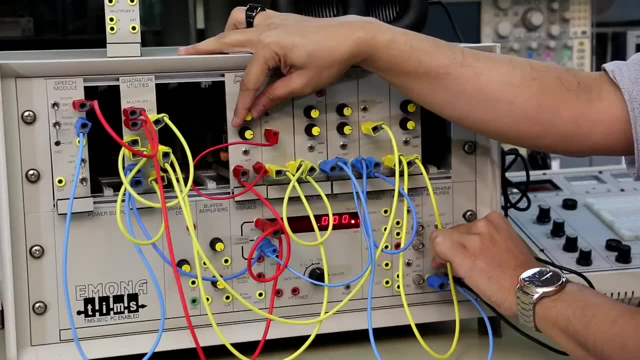 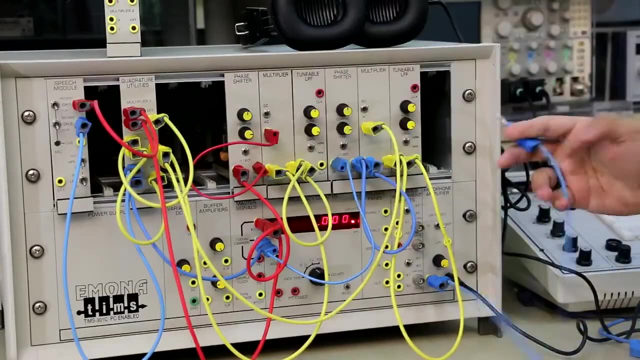 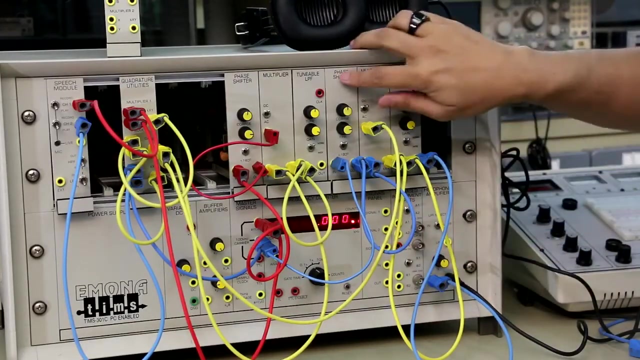 As you can see, there is overlapping between the messages, and the best way to fix that is have a phase shifter that will clear it out. Same thing if you go and listen to the second message, which is here Now, as you can see, the second message is clear, but there. 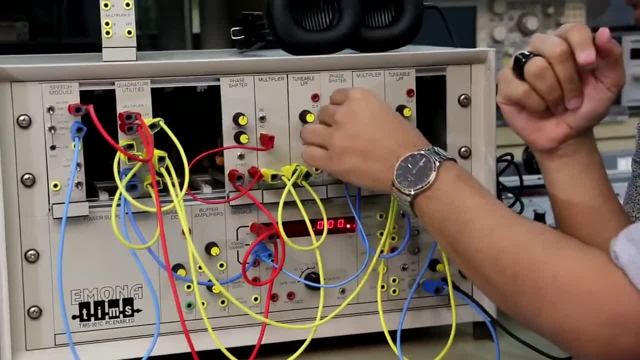 is still interference. So if you want to fix it, you have to do a phase shifting. So if the first message is clear, I have to do a phase shifter. there is still interference from the first message and in order to fix that I have to be careful with my phase here. 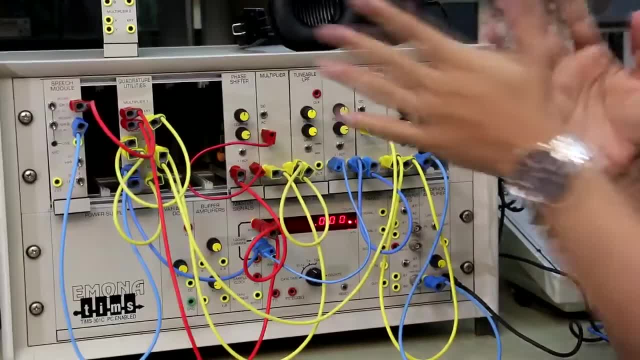 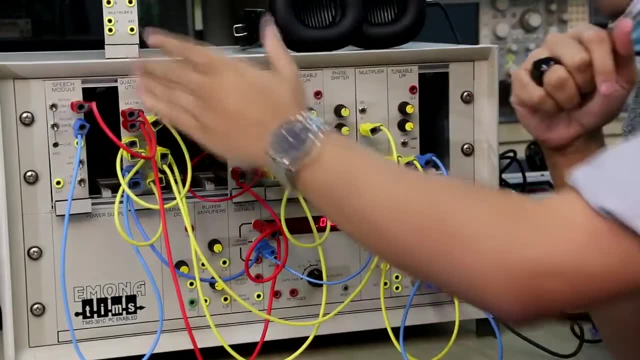 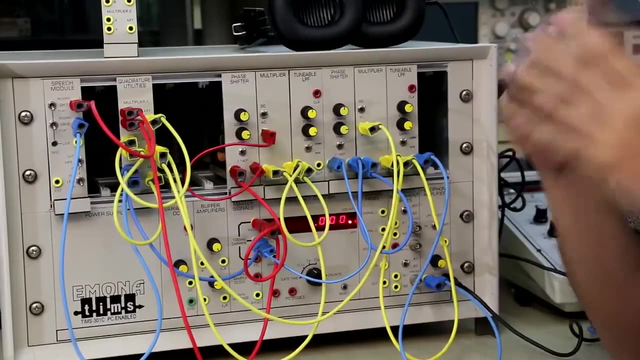 So this is an experiment purpose, But the whole objective is that you are sending two messages, you are getting two messages back. there might be some difference and that is because of the phase difference between the carrier used here and the carrier that is used in the demodulator side. So the more costly equipment you use, that can even fix. 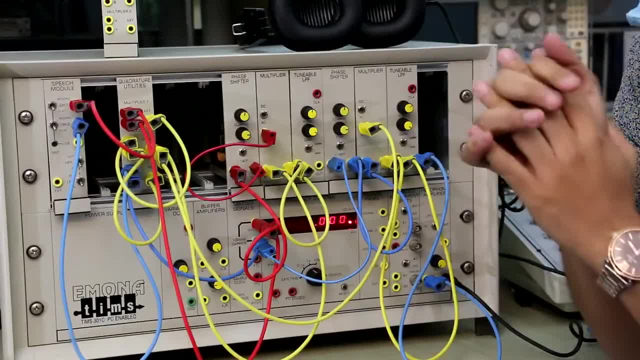 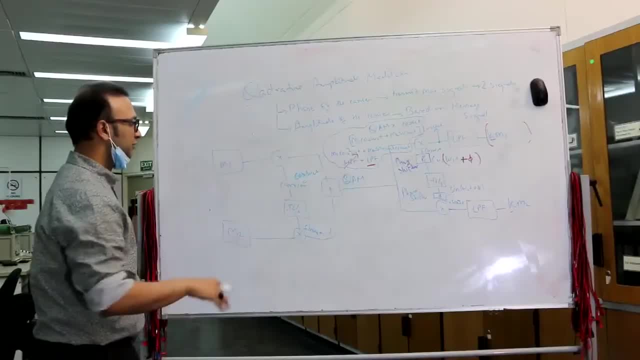 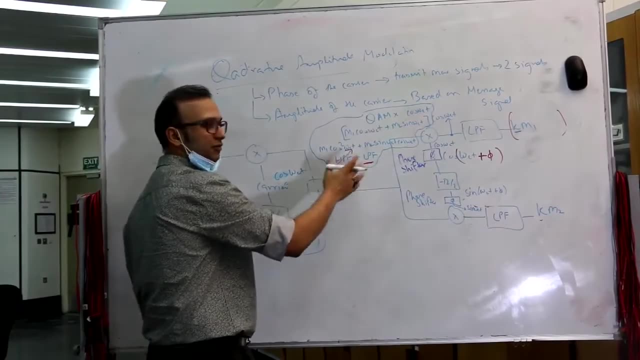 phase, the better or the less interference you will have in the demodulator side. ok, thank you. so in the previous video you have seen how the modulator was made and the demodulator was made and we have seen how we can look at it in time domain and obviously do the 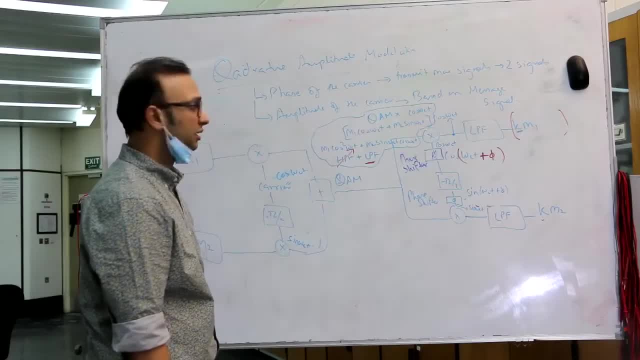 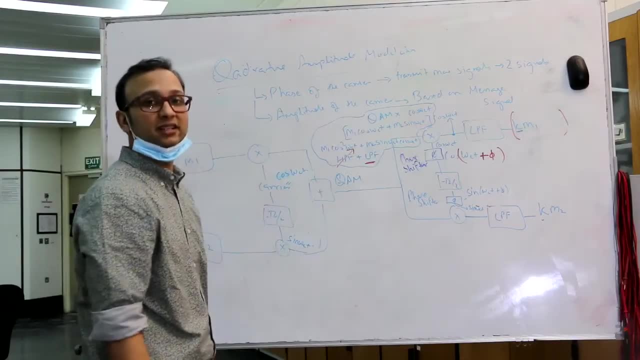 Fourier transform of it to look at it in frequency domain. so I am just going to give you some hints on how it is going to look like and you will be able to relate it to what you have seen earlier. alright, obviously this is clear. why it is called quadrature amplitude? 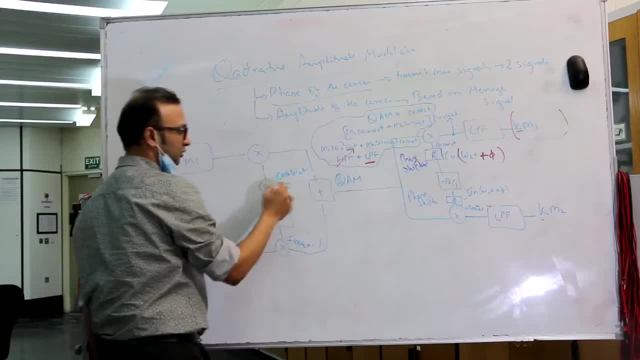 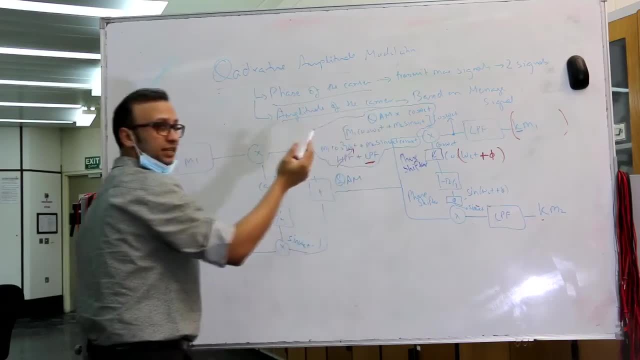 because the phase of the carrier changes. as you can see, there was cosine and it is phase shifted to accommodate the second signal and the amplitude of the carrier is changed based on the message which is evident from the multiplier right. we have two multipliers here. so, if I 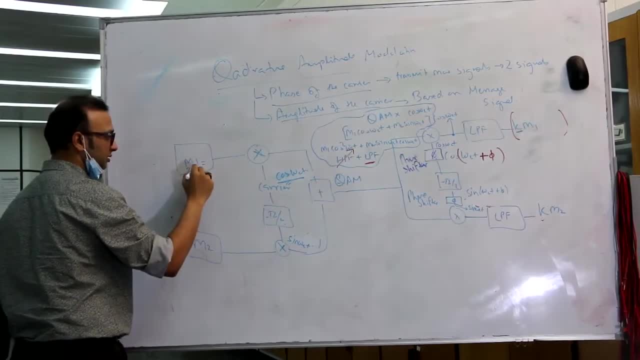 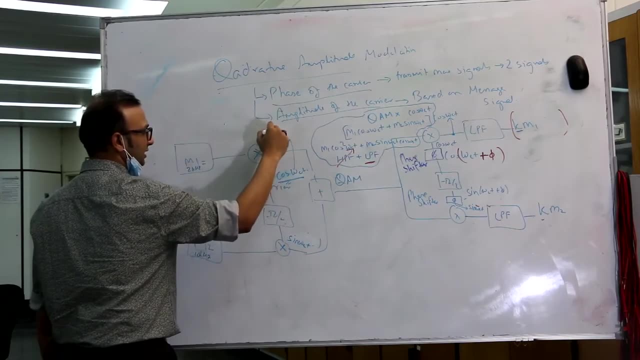 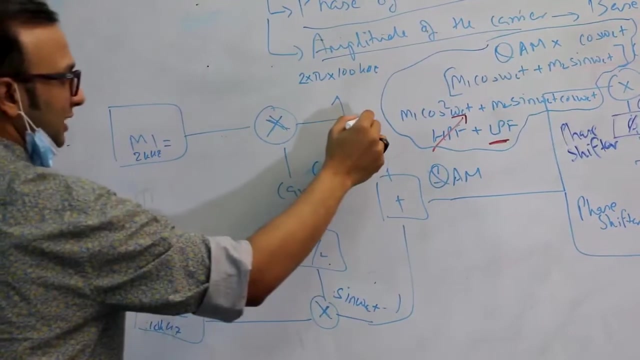 look at this signal and I say: m1 is equal to 2kHz and m2 is equal to 10kHz and the carrier here, omega c, is actually 2 times of pi, times of 100 kilohertz. so the signal that is over here. 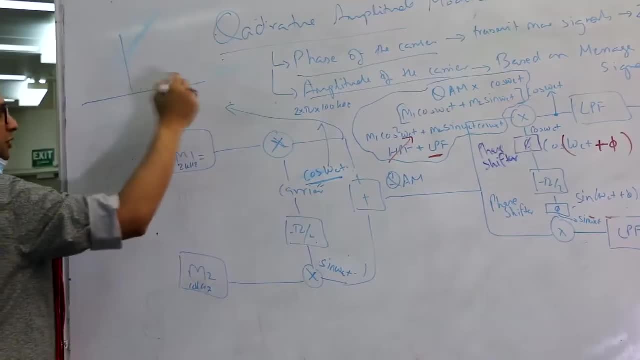 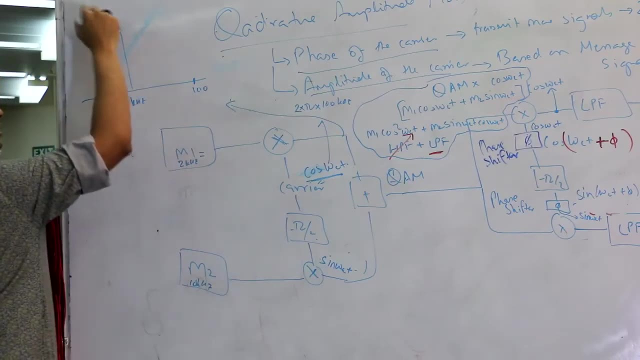 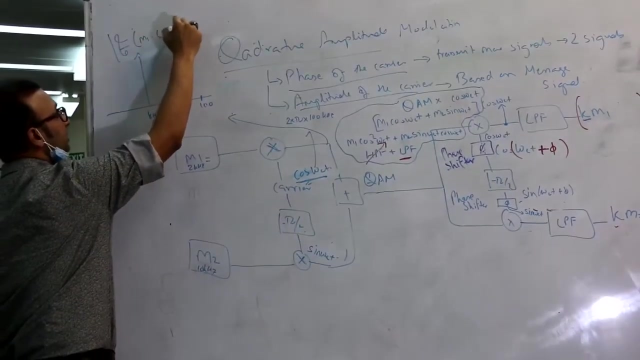 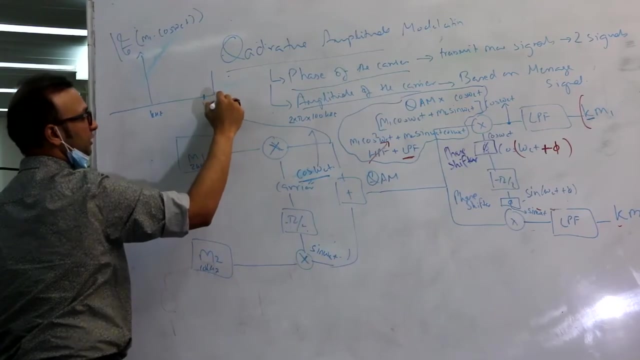 is going to look like i'm sure you know by now- is going to be centered at 100 kilohertz. okay, everything is 100 kilohertz, and we- i'm looking at the magnitude of m1 times cosine, omega ct, right? so it's going to be 100 plus 202 and that's going to be 198 and it's going to be. 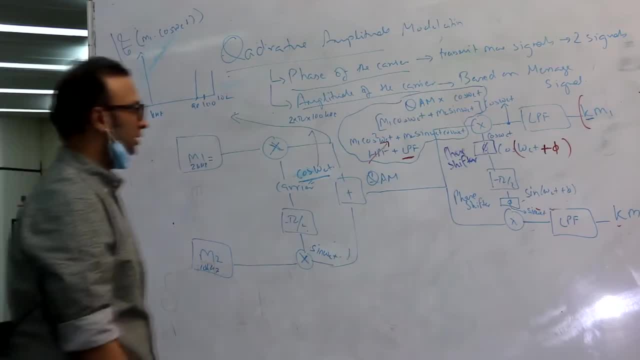 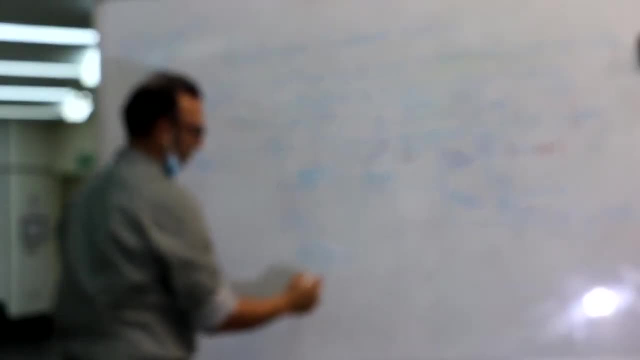 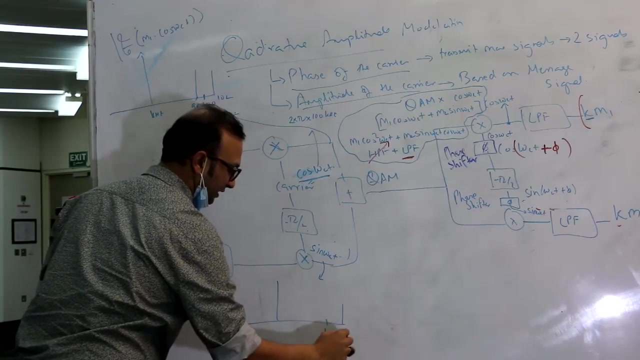 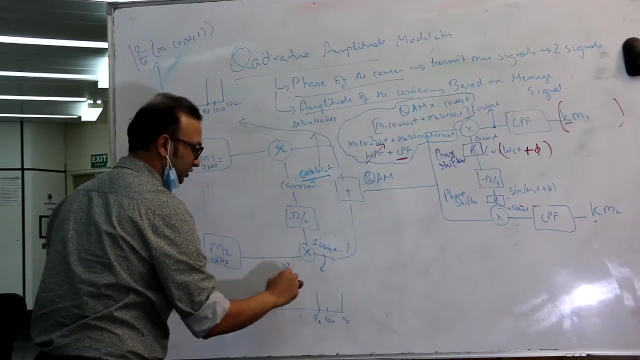 half, and the same thing happens over here. yeah, same thing will happen here. so again, this is 10 kilohertz, so it's going to be 100, so it's going to be 110, so and 90, and this is again fast. fourier transform. magnitude of the fourier transform of. 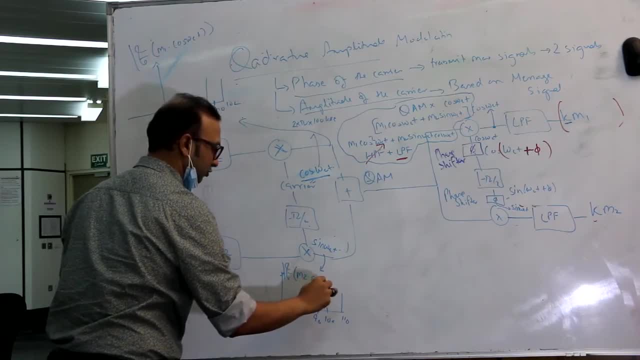 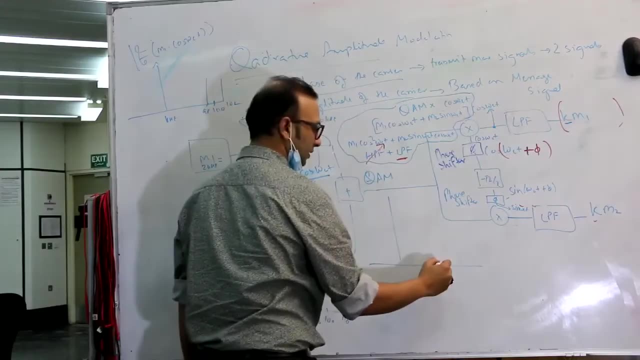 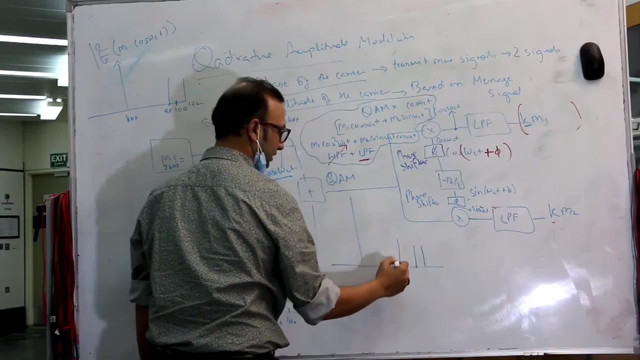 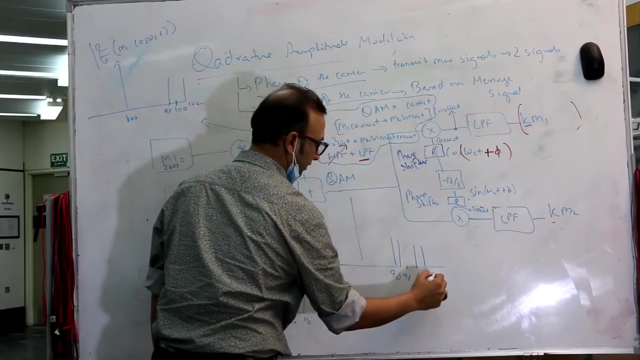 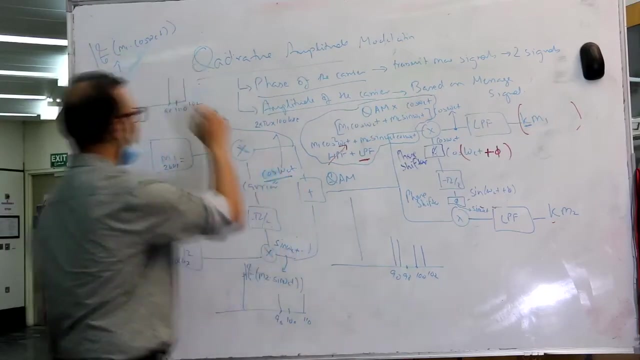 m2 multiplied with sine omega ct, right? so obviously the quam signal is going to look like 100, and then one here: 102, 110, 98 and 90, so this will be one at 90, 98, 100, 102, right? similarly, you can go ahead and look at it afterwards, right? remember, this is what. 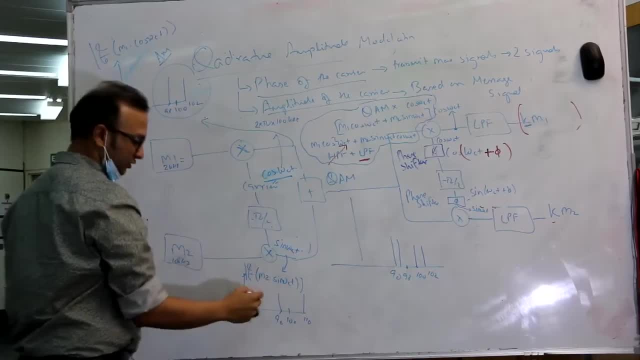 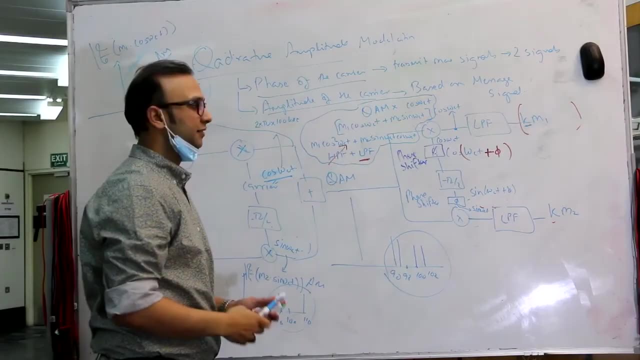 you have seen in am modulation. over here this is also in am modulation and over here it's actually summation of two am signals. all right, thank you.